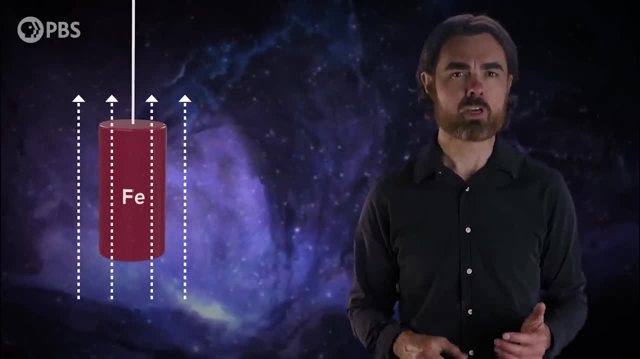 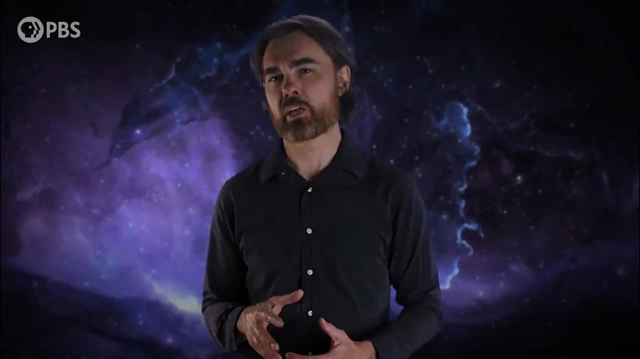 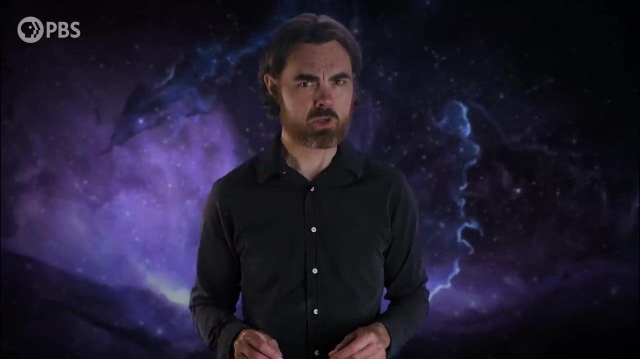 iron from a thread and switch on a vertical magnetic field, The cylinder immediately starts rotating with a constant speed. At first glance, this appears to violate conservation of angular momentum, because there was nothing spinning to start with. Except there was, Or at least there sort of was. The external magnetic field magnetized the iron, causing 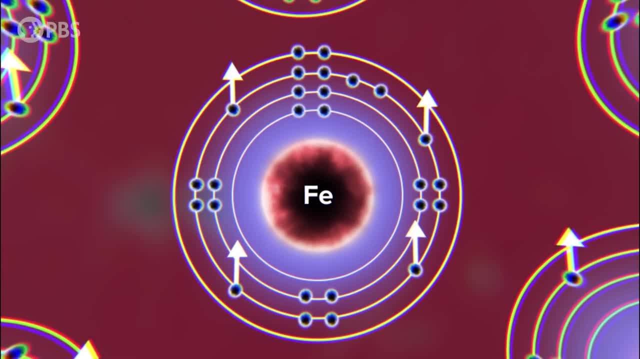 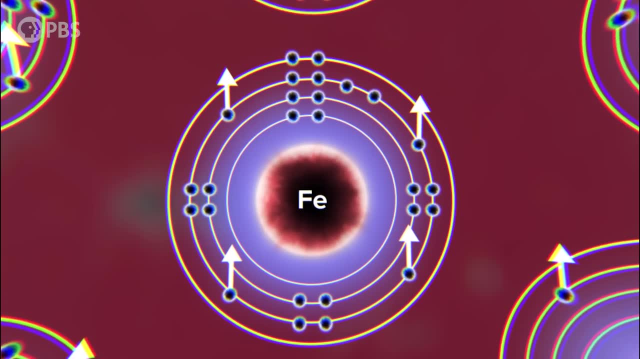 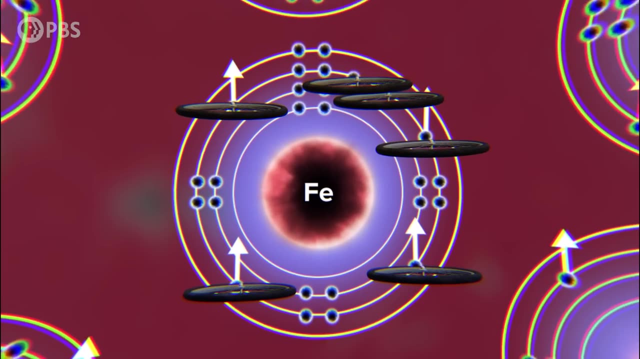 the electrons in the iron's outer shells to align their spins. Those electrons are acting like tiny bicycle wheels and their shifted angular momentum is compensated by rotating the cylinder. That explanation makes sense if we imagine the electrons like spinning bicycle wheels or like spinning anything Which might sound fine, because electrons do have this property that we 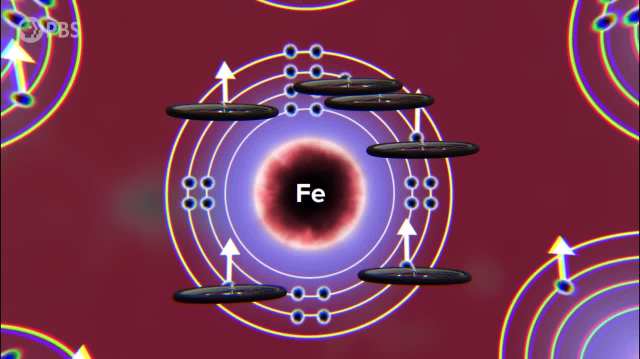 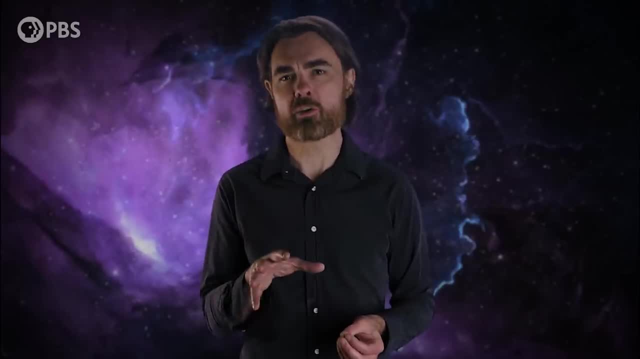 call spin, But there's a huge problem. Electrons are definitely not spinning like bicycle wheels, and yet they do seem to possess a very strange type of angular momentum that somehow exists without classical rotation. In fact, the spin of the electron is far more fundamental. 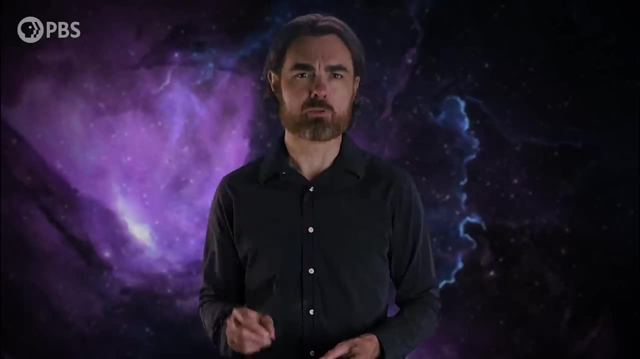 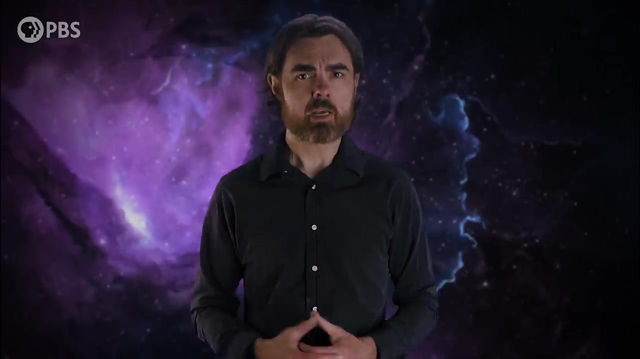 than simple rotation. It's a quirk quantum property of particles like mass or the various charges. But it doesn't just cause magnets to move in funny ways. It turns out that quantum spin is a manifestation of a much deeper property of particles. 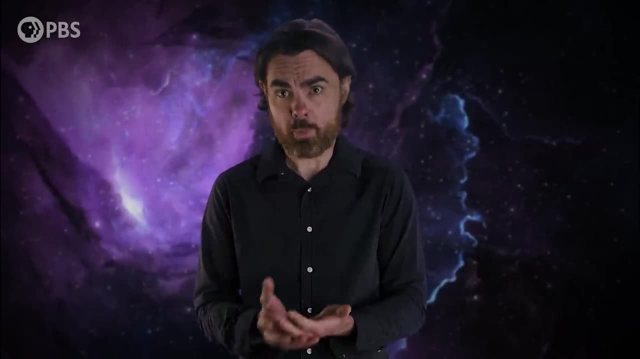 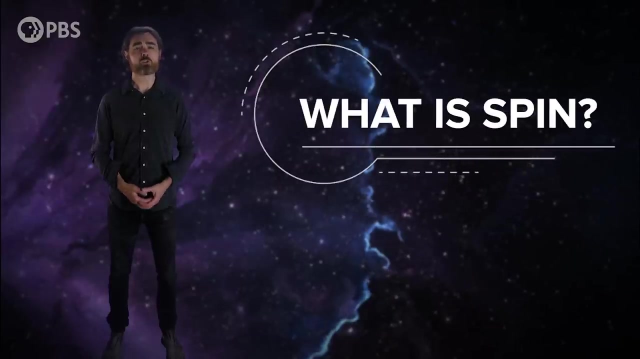 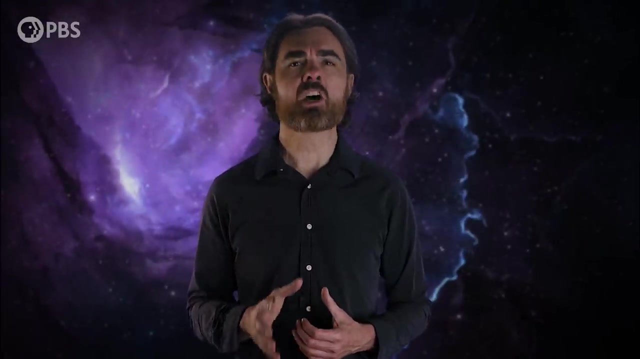 A property that is responsible for the structure of all matter. We'll unravel all of that over a couple of episodes, but today I want to talk about what spin really is and get a little closer to understanding this weird property of nature. The experiment with the iron cylinder is called the Einstein-De Haas effect, first performed 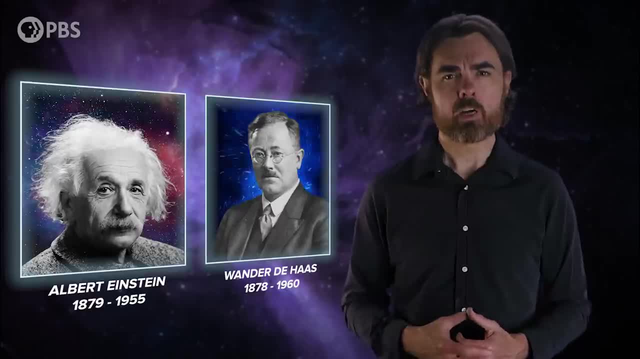 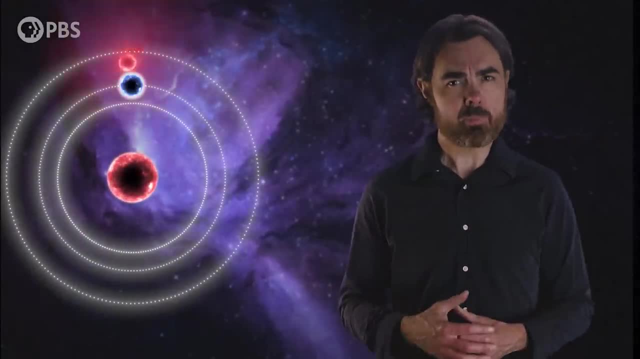 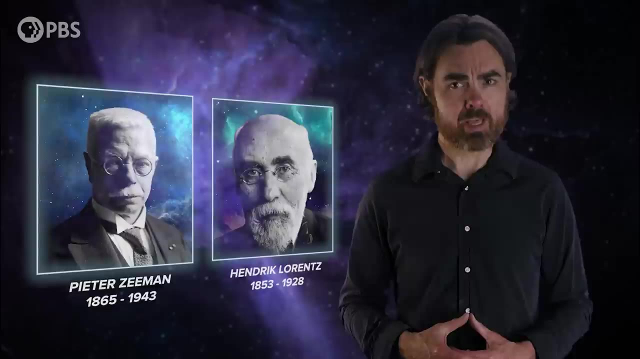 by well Einstein and De Haas in 1915.. It wasn't the first indication of the spin-like properties of electrons That came from looking at the specific wavelengths of photons emitted when electrons jumped between energy levels in atoms. Peter Zeeman, working with the great Heinrich Lorentz in the Netherlands, found that these 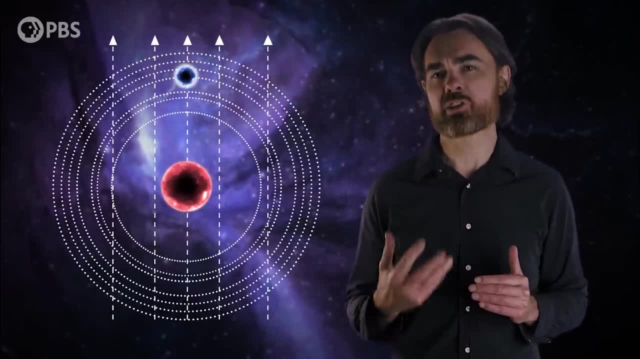 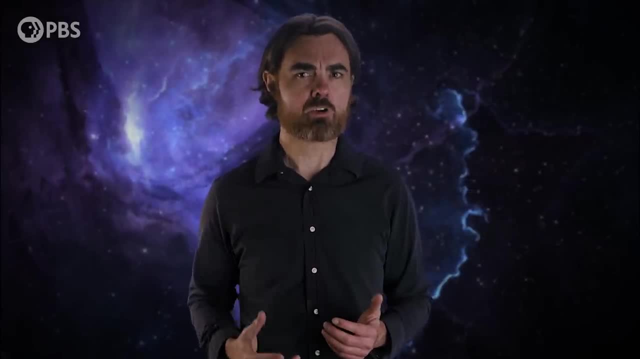 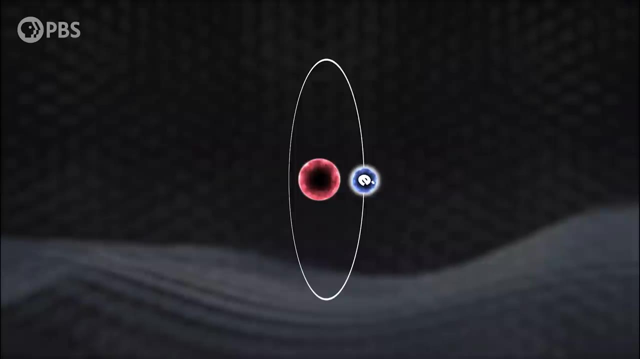 energy levels tend to split when atoms are put in an external magnetic field. This Zeeman effect was explained by Lorentz himself with the ideas of classical physics. If you think of an electron as a ball of charge moving in a circle around the atom, that motion. 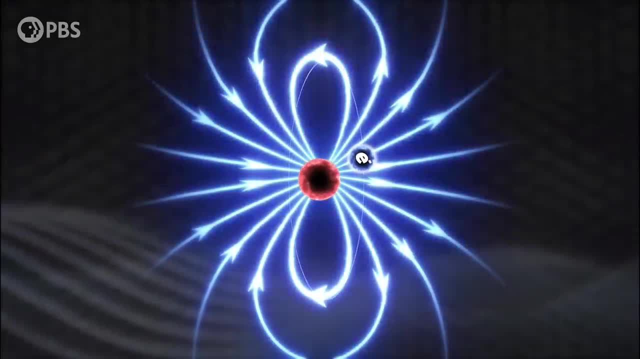 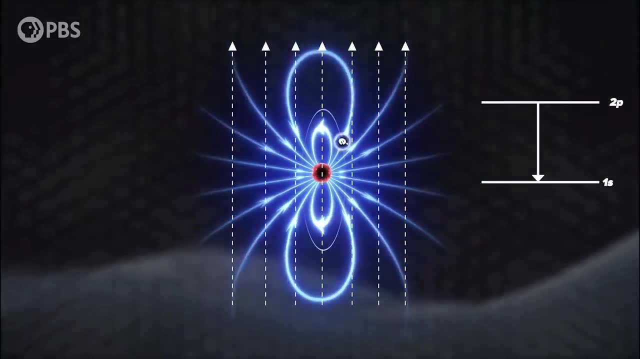 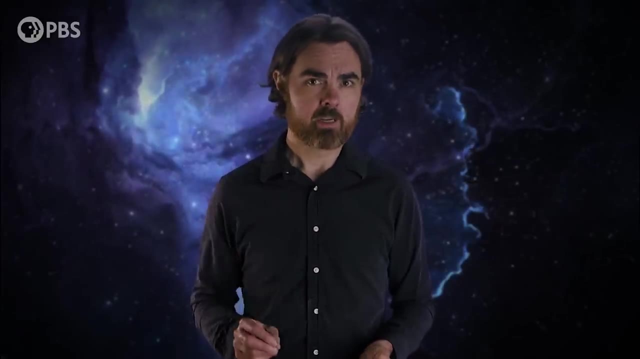 leads to a magnetic moment, a dipole magnetic field like a tiny bar magnet. The different alignments of that orbital magnetic field relative to the external field turns one energy level into three. Well, sounds reasonable. But then came the anomalous Zeeman effect. 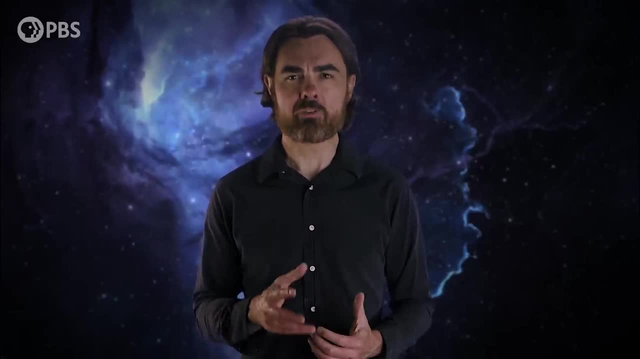 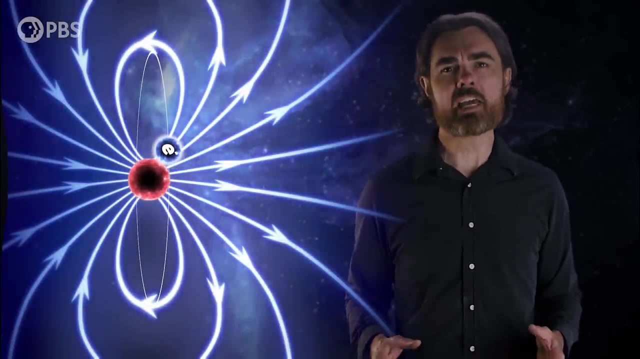 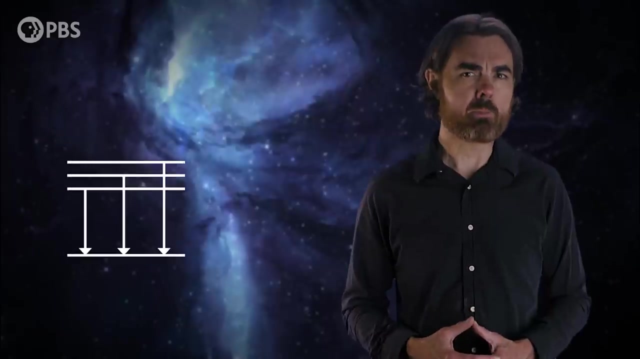 In some cases, the magnetic field causes energy levels to split even further, for reasons that were at the time a complete mystery. One explanation that sort of works is to say that each electron has its own magnetic moment. By itself it acts like a tiny bar magnet, so you have the alignment of both the orbital 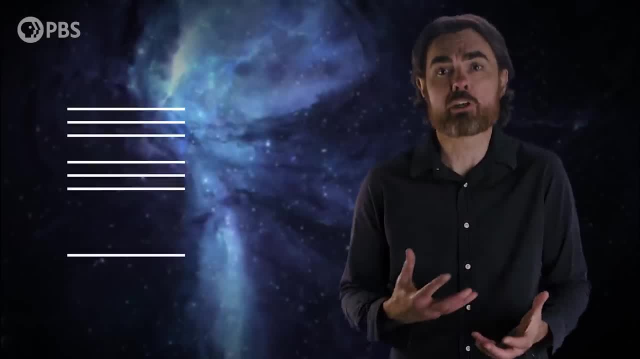 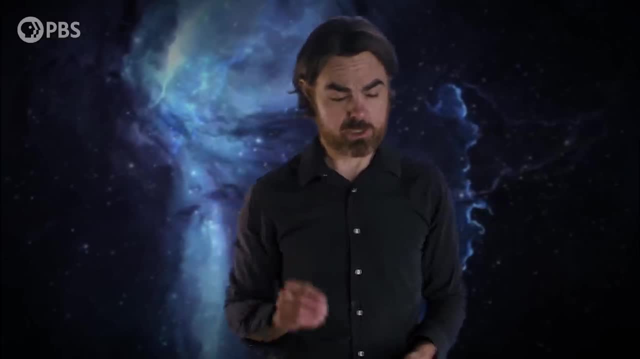 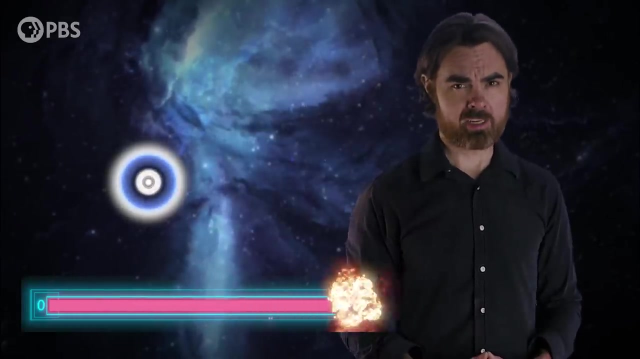 magnetic moment and the electron's internal moment contributing new energy levels. But for that to make sense, we really need to think of electrons as balls of spinning charge. For example, in order to produce the observed magnetic moment, they'd need to be spinning faster than the speed of light. 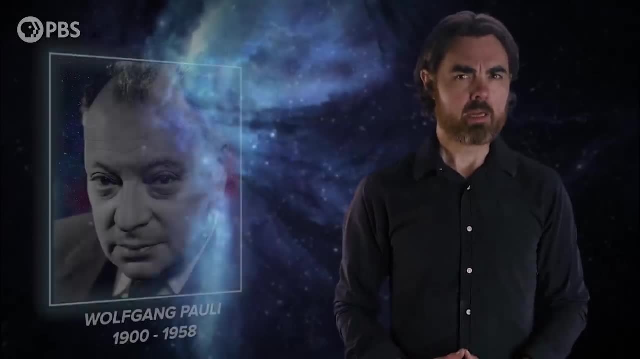 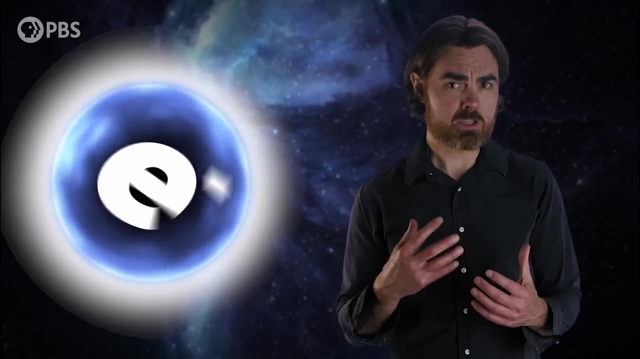 This was first pointed out by the Austrian physicist Wolfgang Pauli. He showed that if you assume electrons have the maximum possible size given by the best measurements of the day, then their surfaces would have to be moving faster than light to give the required angular momentum. 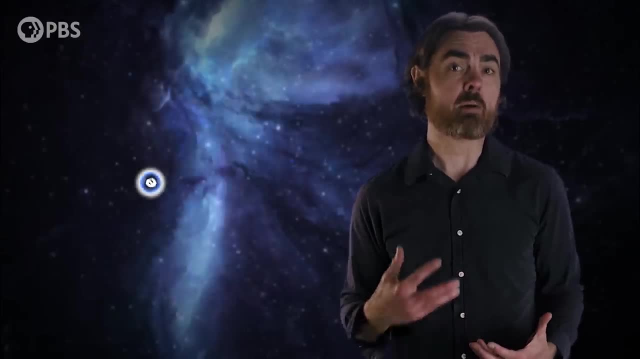 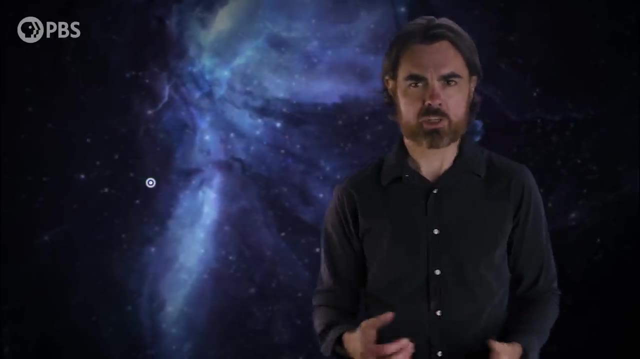 And that's assuming the electrons even have a size. As far as we know, they are point-like. They have zero size, Which would make the idea of classical physics, Classical angular momentum, even more nonsensical. Pauli rejected the idea of associating such a classical property, like rotation, to the 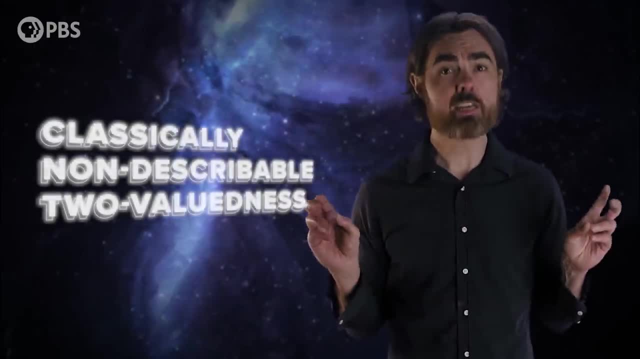 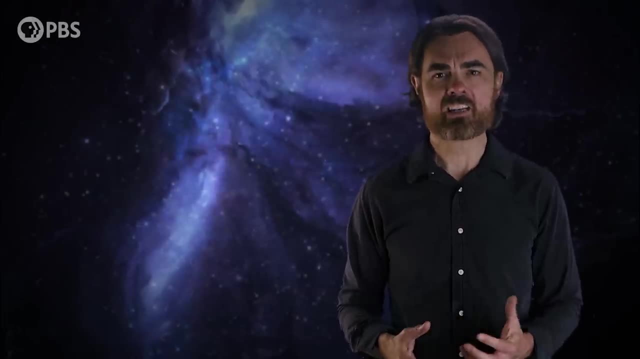 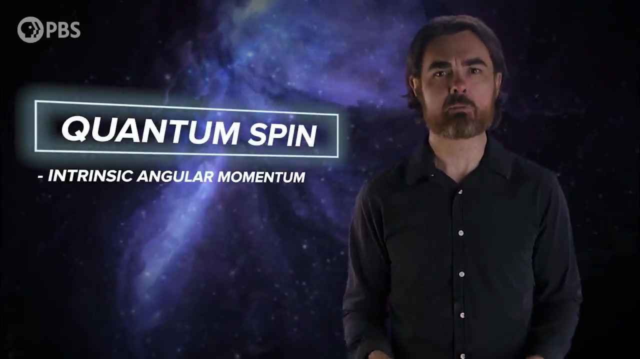 electron, instead insisting on calling it classically nondescribable two-valuedness. OK, so electrons aren't spinning, but somehow they act like they have angular momentum, And this is how we think about quantum spin. now, It's an intrinsic angular momentum that plays into the conservation of angular momentum. 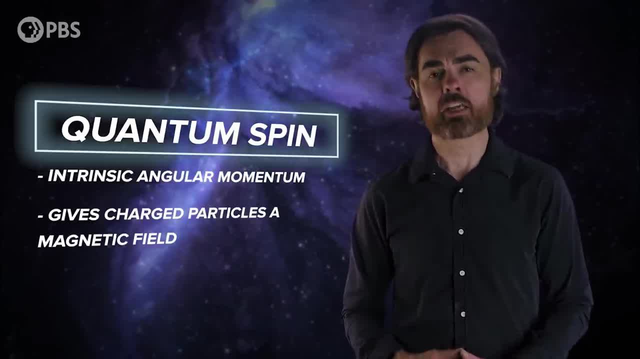 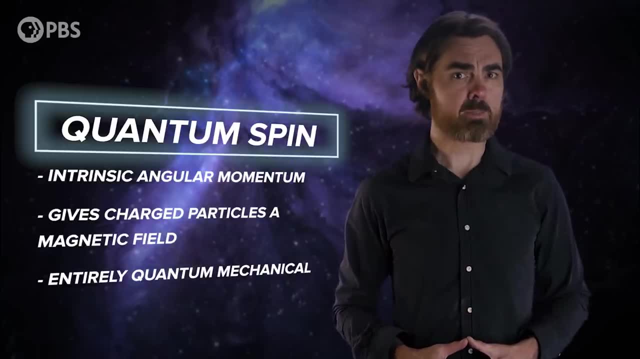 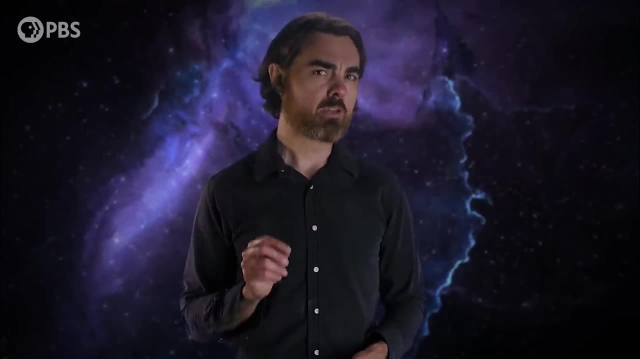 like in the Einstein-De Haas effect, And it also gives electrons a magnetic field, And electron spin is an entirely quantum mechanical property and has all the weirdness you'd expect from the weirdest of theories. But before we dive into that weirdness, let me give you one more experiment that reveals: 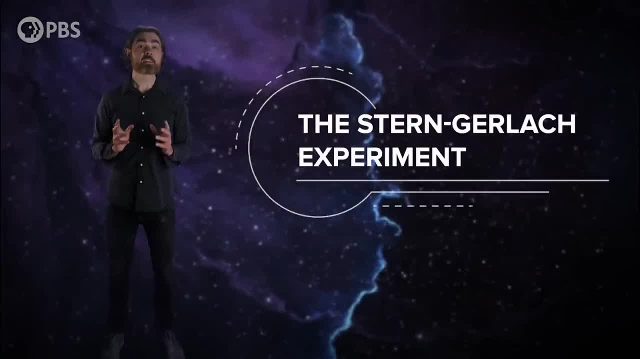 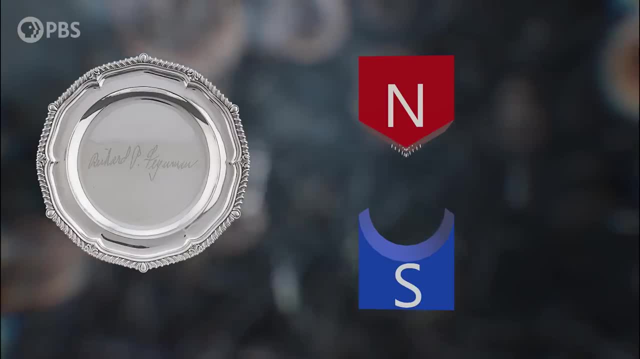 the magnetic properties that result from spin. This is the Stern-Gerlach experiment, proposed by Otto Stern in 1921 and performed by Walter Gerlach a year later. In it, The atoms are fired through a magnetic field with a gradient. 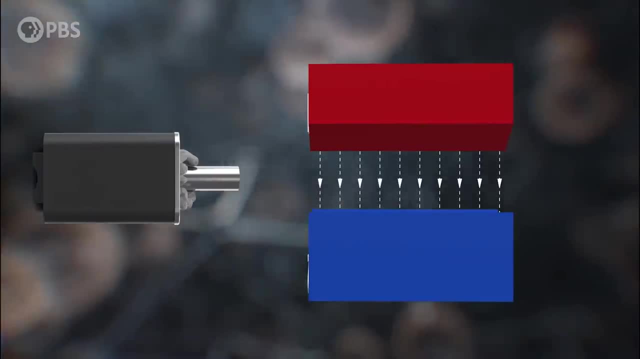 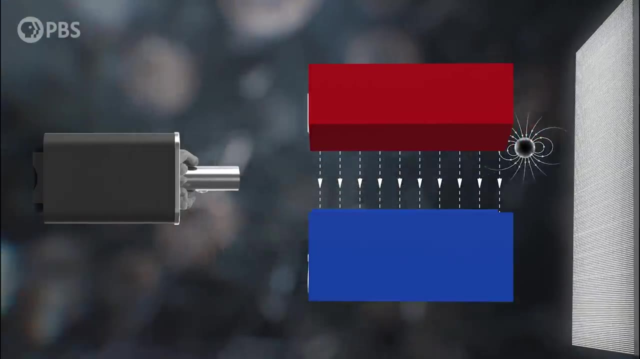 In this example, stronger towards the north pole above and getting weaker going down. A lone electron in the outer shell of the silver atoms grants those atoms a magnetic moment. That means the external magnetic field induces a force on the atoms that depends on the directions. 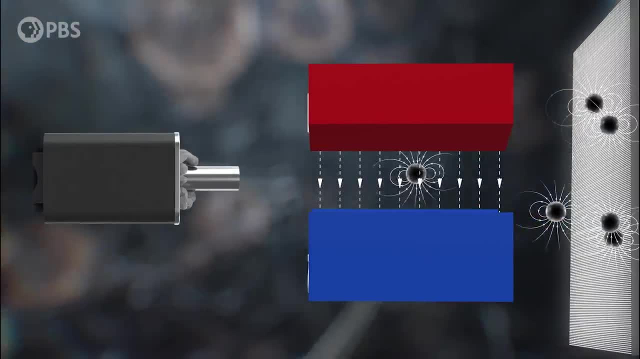 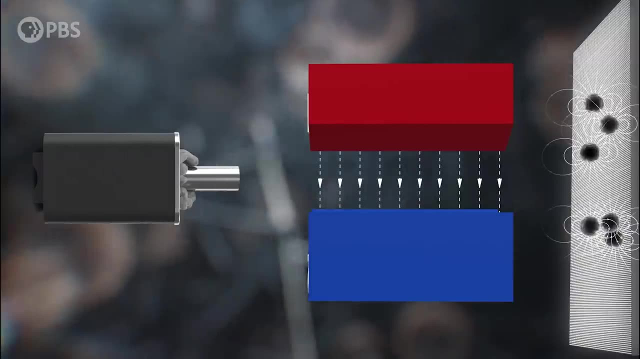 that these little magnetic moments are pointing relative to that field. Those that are perfectly aligned with the field will be deflected by the most, either up or down. If these were classical dipole fields, like actual tiny bar magnets, then the ones that were only partially aligned with the external field should be deflected by less. 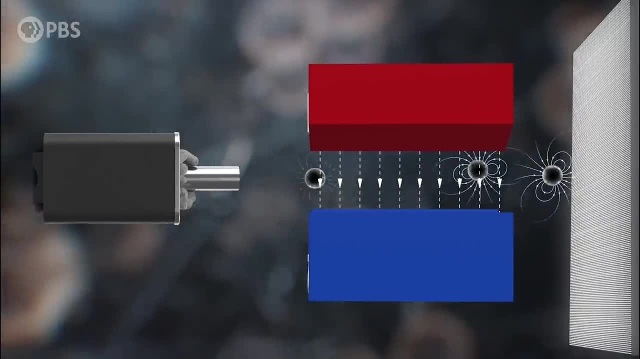 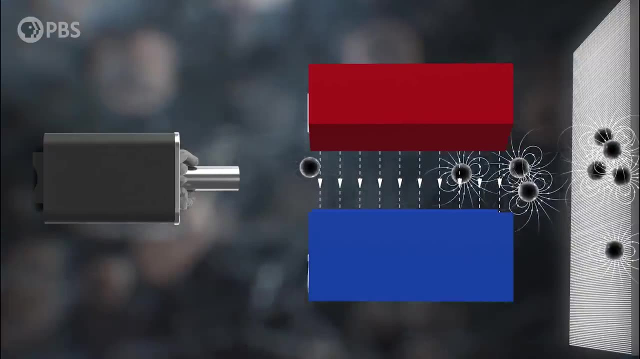 So a stream of silver atoms with randomly aligned magnetic moments is sent through the magnetic field. You might expect a blur of points where the silver atoms hit the detector screen, some deflected up or down by the maximum, but most deflected somewhere in between. due to all, 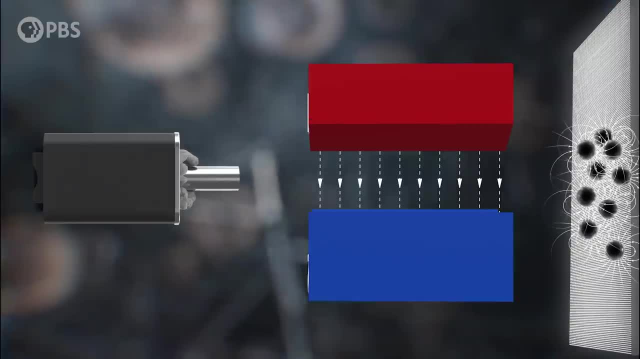 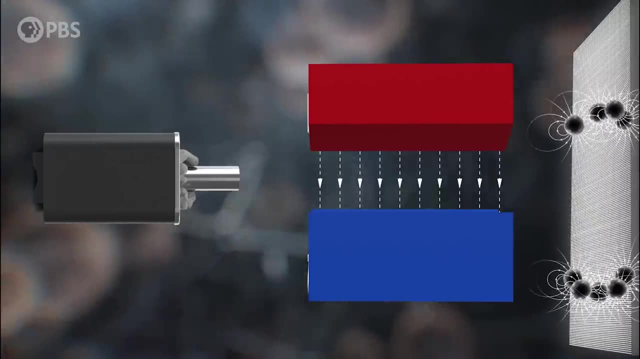 the random orientations, But that is not what's observed. Instead, the atoms hit the screen in only two spots, corresponding to the most extreme deflections. Let's keep going. What if we remove the screen and bring the beam of atoms back together? 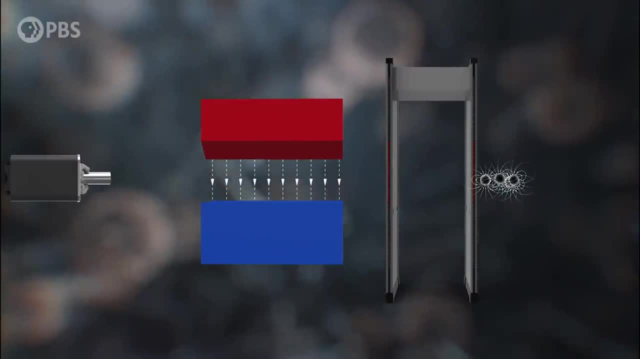 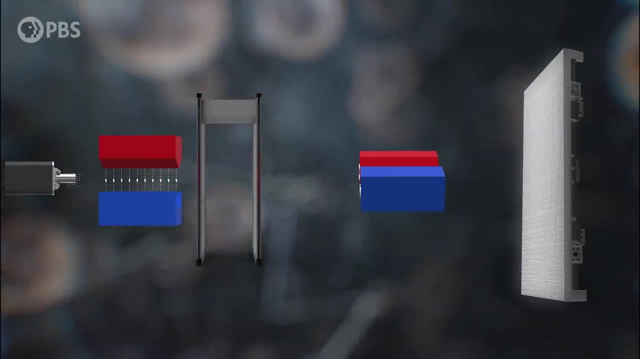 Now we know that the electrons have to be aligned only up or down, Let's send them through a second set of stern Gerlach magnets, but now they're oriented horizontally. Classical dipoles that are at 90 degrees to the field. 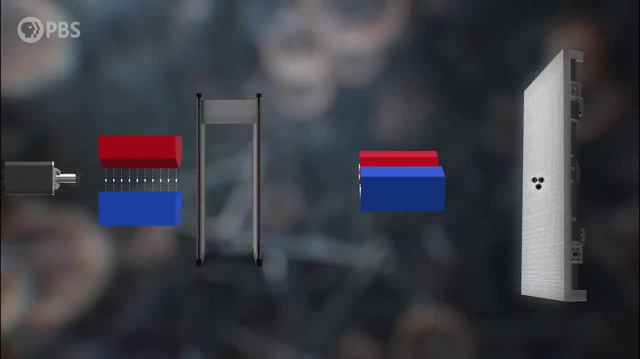 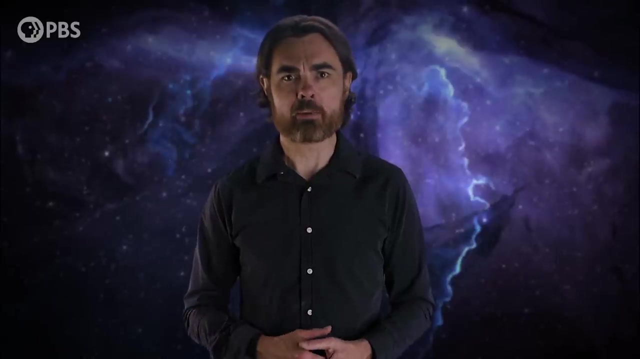 No force whatsoever. But if we put our detector screen we see that the atoms again land in two spots, now also oriented horizontally. So not only do electrons have this magnetic moment without rotation, but the direction of the underlying magnetic moment is fundamentally quantum. 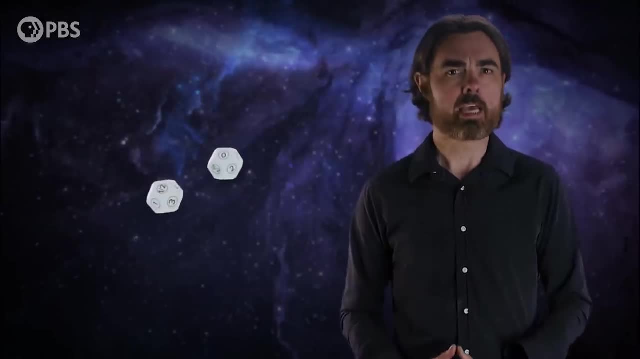 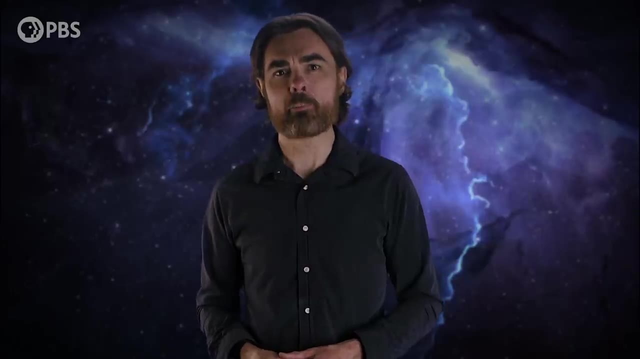 The direction of this spin property is quantized. It can only take on specific values, and that direction depends on the direction in which you choose to measure it. Here we see an example of Pauli's too-valuedness manifesting as something like the direction. 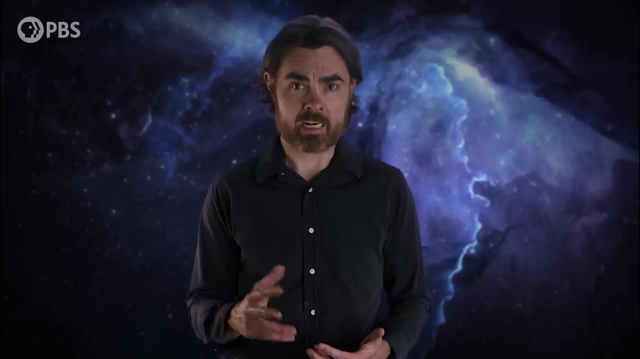 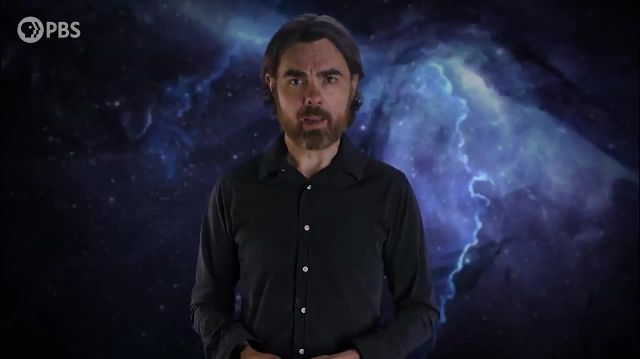 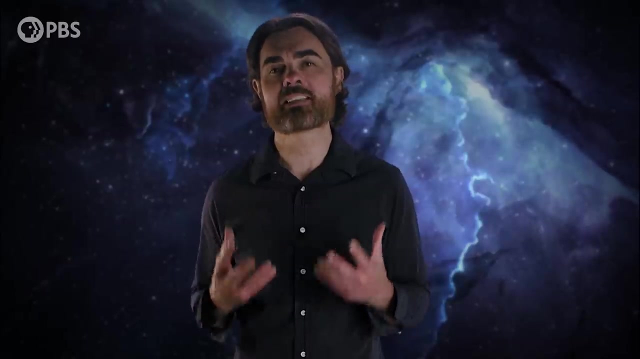 of a rotation axis or the north-south pole of the magnetic dipole. But actually this too-valuedness is far deeper than that. To understand why we need to see how spin is described in quantum mechanics, It was again Pauli who had the first big success here. 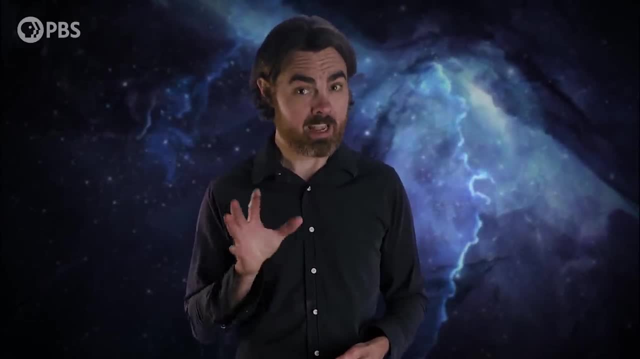 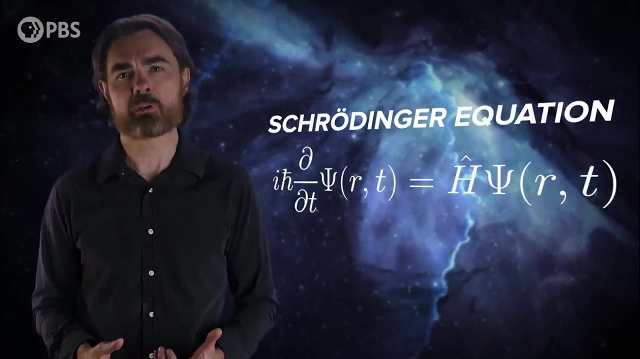 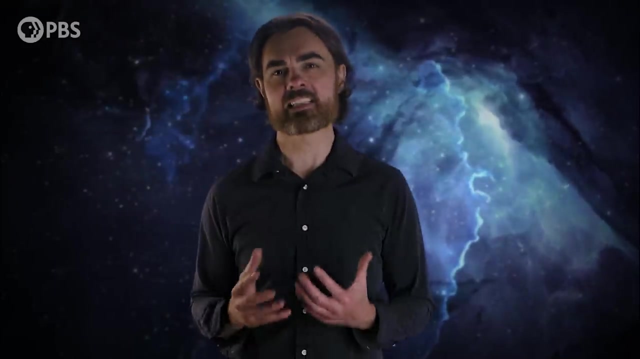 By the mid 1920s, physicists were very excited about a brand new tool. new tool they'd been given the Schrodinger equation. This equation describes how quantum objects behave as evolving distributions of probability, as wave functions. It was proving amazingly successful at describing some aspects of the subatomic world. but the equation as 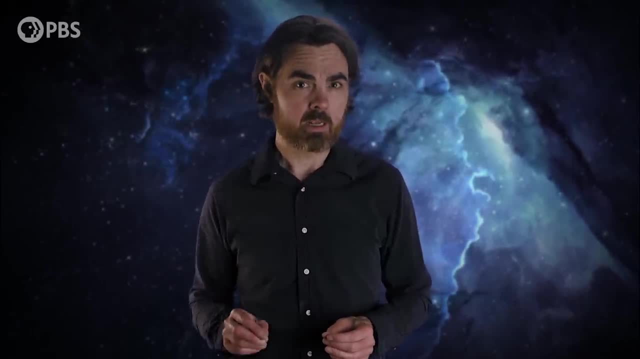 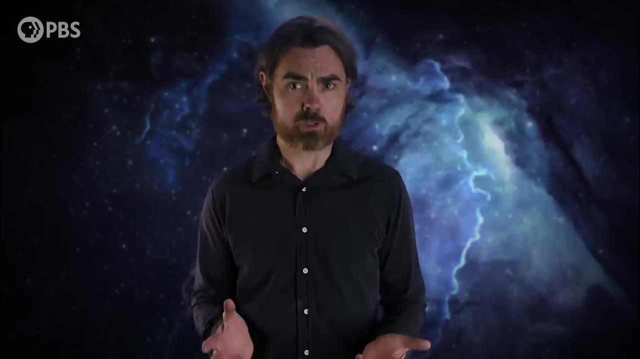 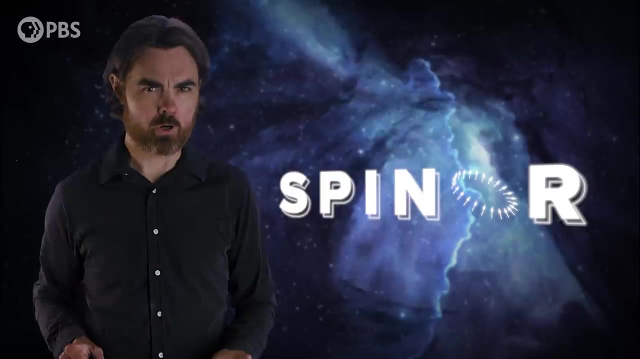 Schrodinger first conceived it did not include. spin Pauli managed to fix this by forcing the wave function to have two components. motivated by this ambiguous, too-valuedness of electrons, The wave function became a very strange mathematical object called a spinor. 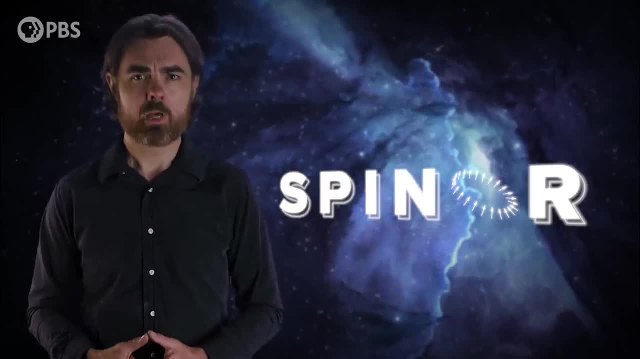 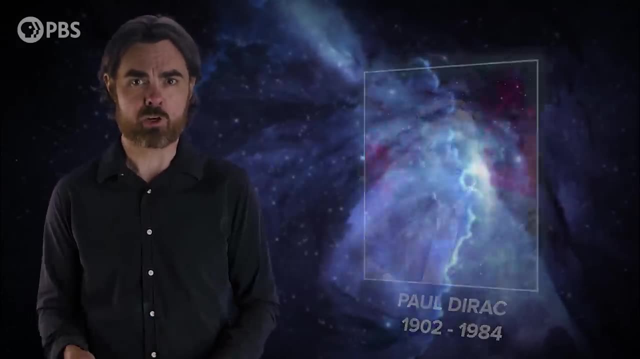 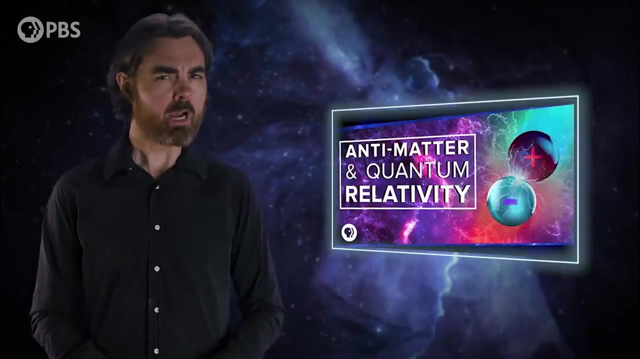 which had just been invented. a decade prior, And just one year after Pauli's discovery, Paul Dirac found his own, even more complete fix of the Schrodinger equation, In this case to make it work with Einstein's special theory of relativity, something we've discussed before. Dirac wasn't. 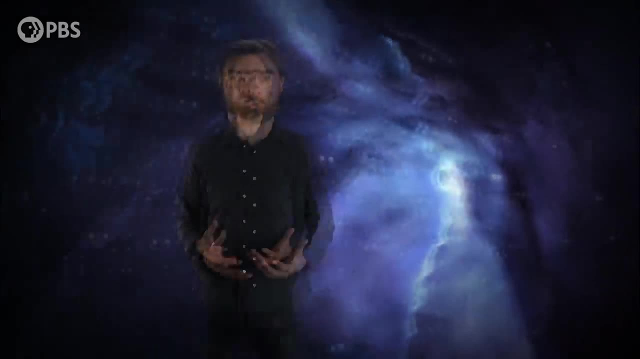 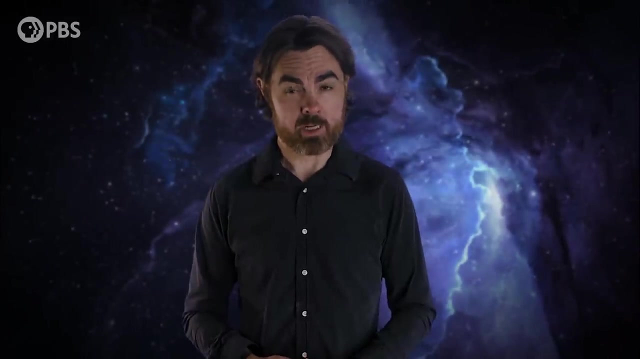 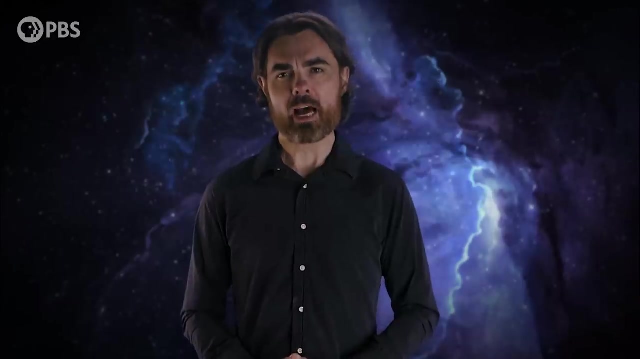 even trying to incorporate spin, but the only way the equation could be derived was using spinors. Now, spinors are exceptionally weird and cool and really deserve their own episode, But let me say a couple of things to give you a taste. They describe particles that have very strange rotation. 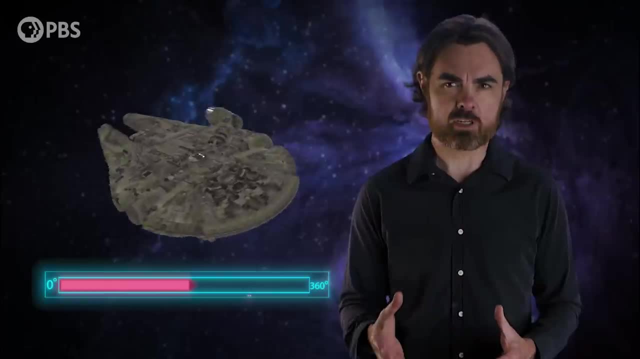 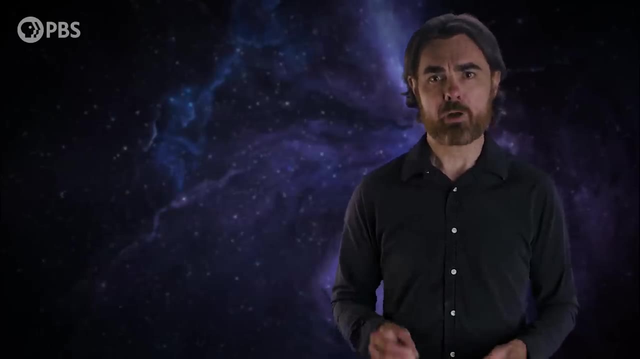 properties For familiar objects. a rotation of 360 degrees gets it back to its starting point. That's also true of vectors, which are just arrows pointing in some space, but for a spinner you need to rotate it twice or 720 degrees to get it back to its starting point. 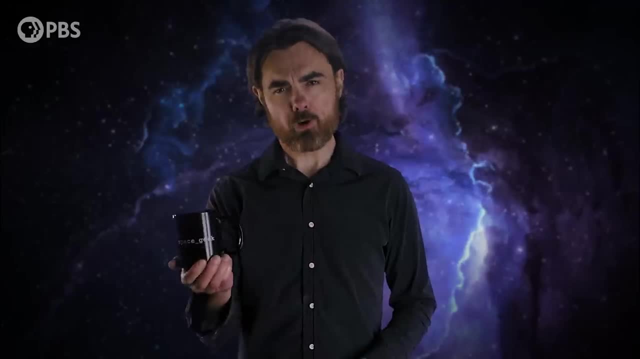 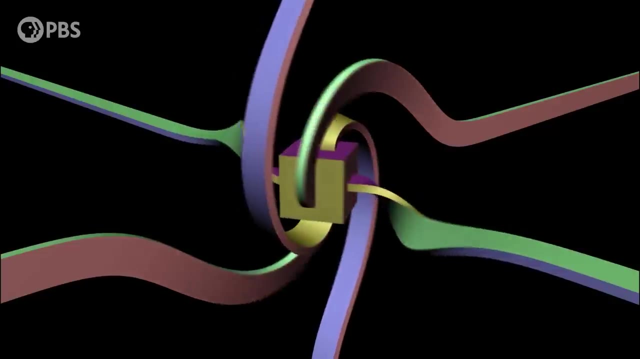 Here's an example of spinner-like behavior. If I rotate this mug without letting go, my arm gets in a twist. but a second rotation untwists me. We can also visualize this with a cube attached to nearby walls by ribbons. If we rotate the cube, 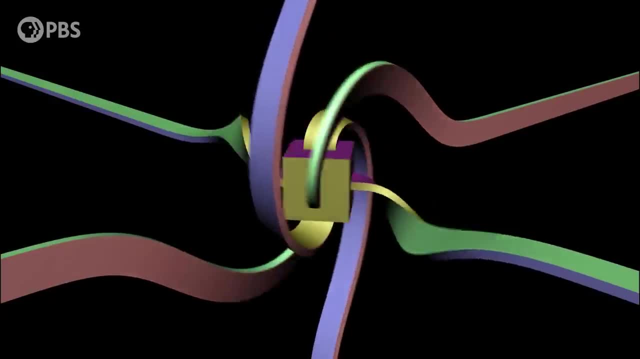 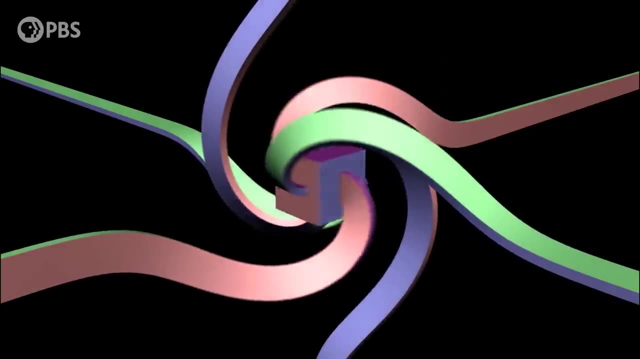 by 360 degrees. the cube itself is back to the starting point, but the ribbons have a twist compared to how they started. Amazingly, if we rotate another 360, not backwards, but in the same direction- we get the whole system back to its starting point. 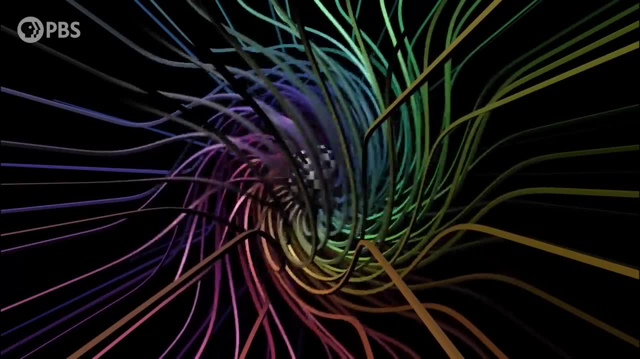 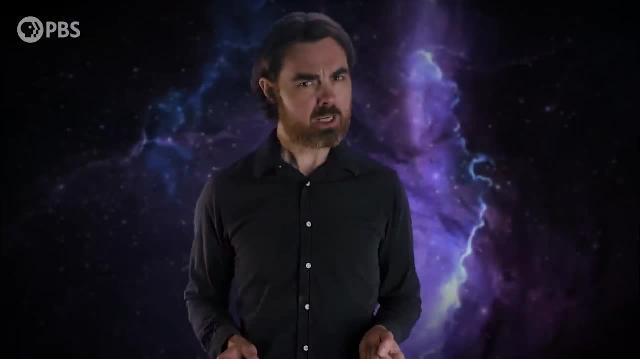 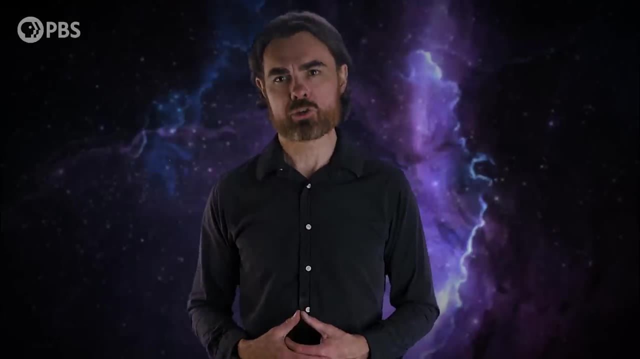 Another thing to notice is that the cube can rotate any number of times with any number of ribbons attached, and it never gets tangled. So think of electrons as being connected to all other points in the universe by invisible strands. One rotation causes a twist, two brings it back to normal. 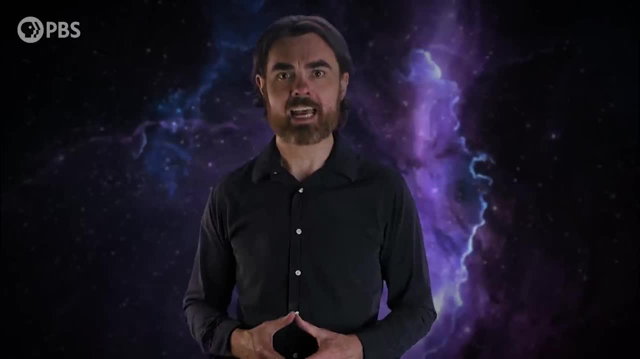 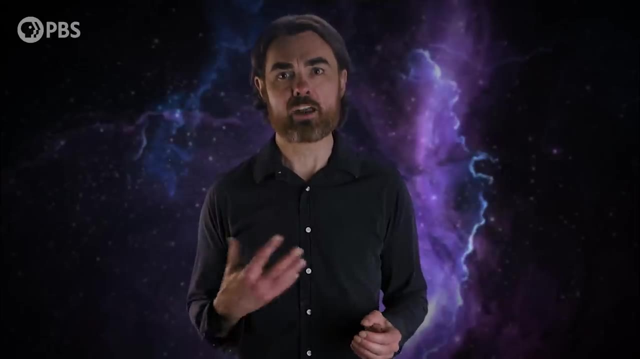 To get a little more technical, the spinor wave function has a phase that changes with orientation angle and a 360 degree rotation pulls it out of phase compared to the starting point. To get some insight into what spin really is, think for a second. not about angular momentum. 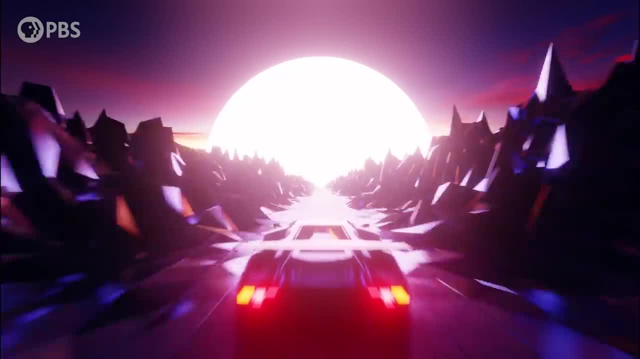 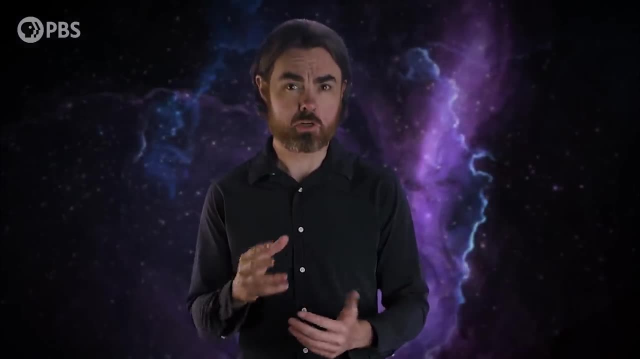 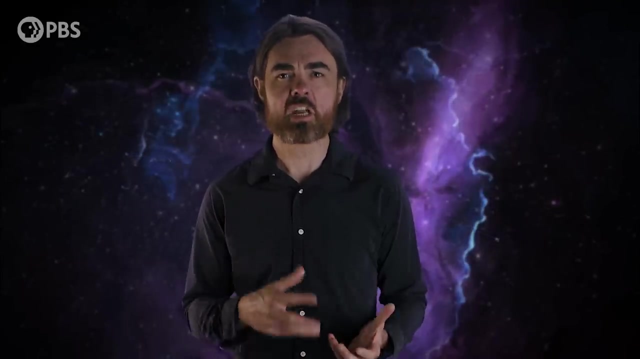 but about regular or linear momentum. A particle's momentum is fundamentally connected to its position By Noether's theorem. the invariance of the laws of motion to changes in coordinate location gives us the law of conservation of momentum. For related reasons, in quantum mechanics, position and momentum are conjugate variables. 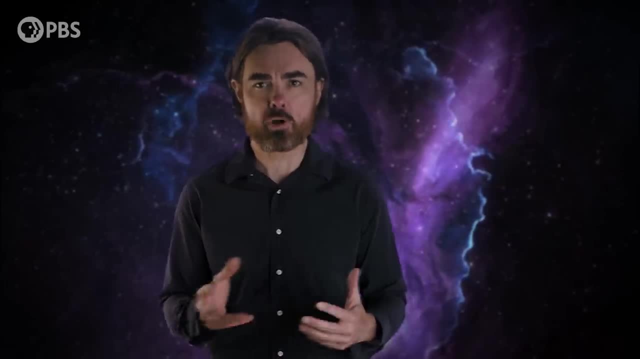 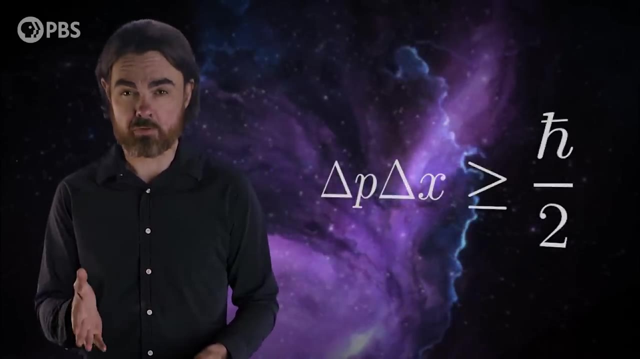 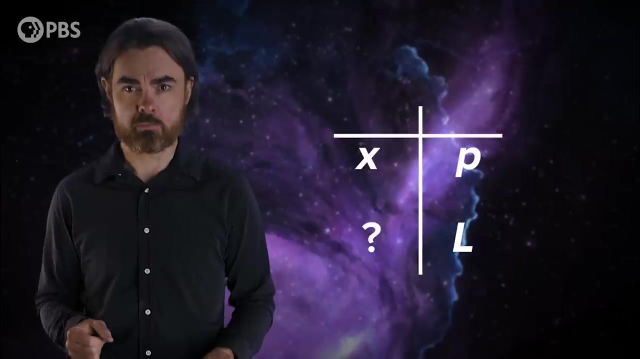 meaning you can represent a particle wave function in either of these properties And by Heisenberg's uncertainty principle, increasing your knowledge of one means increasing the unknowability of the other. If position is the companion variable of momentum, what's the companion of angular momentum? 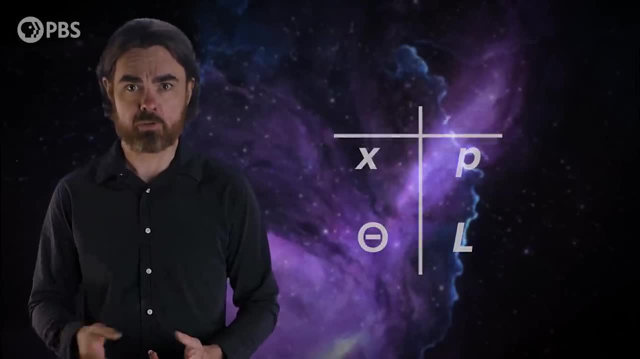 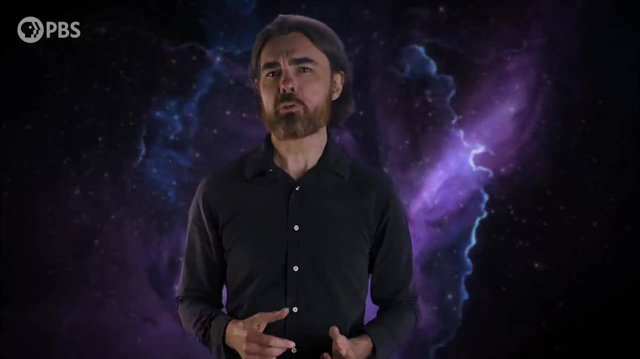 Well, it's angular position, In other words the orientation of the particle. So one way to think about the angular momentum of an electron is not from classical rotation, but rather from the fact that they have a rotational degree of freedom which leads to a conserved quantum. 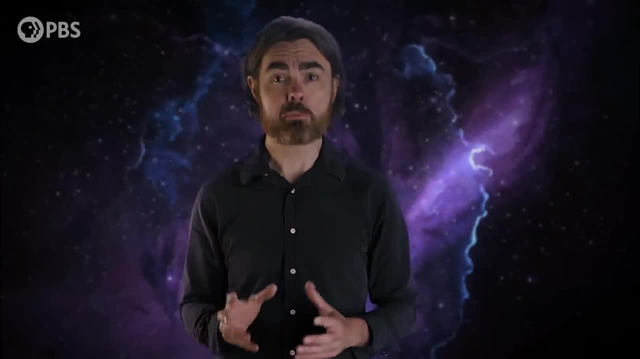 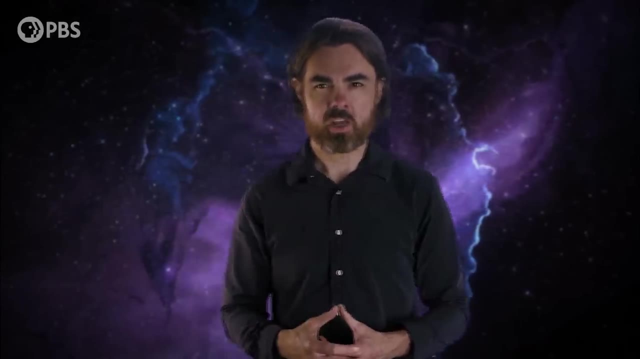 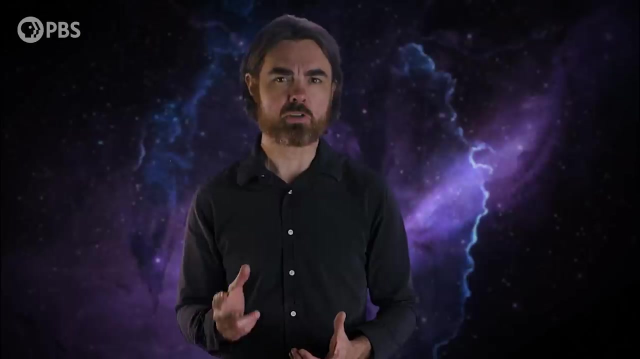 In other words, the angular momentum of an electron is not the quantity associated with that. They have undefined orientations, but perfectly defined angular momentum. Some physicists think that spin is more physical than this. Hans Ohanian, author of one of the most used quantum textbooks, has shown that you can derive. 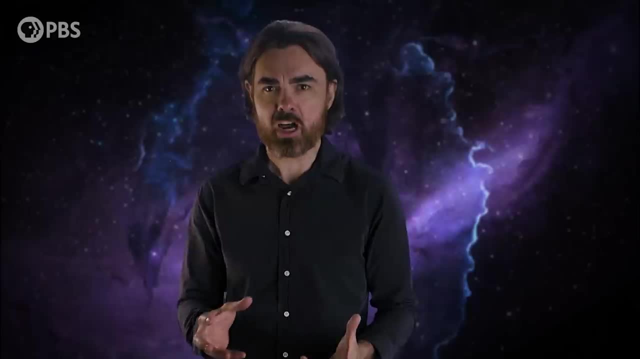 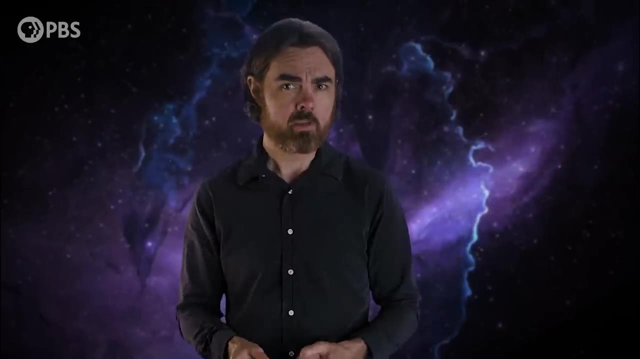 the right values of the electron spin, angular momentum and magnetic moment by looking at the energy and charge currents in the so-called Dirac field, That's, the quantum field surrounding the electron, implying that even if the electron is point-like, its angular momentum can arise from. 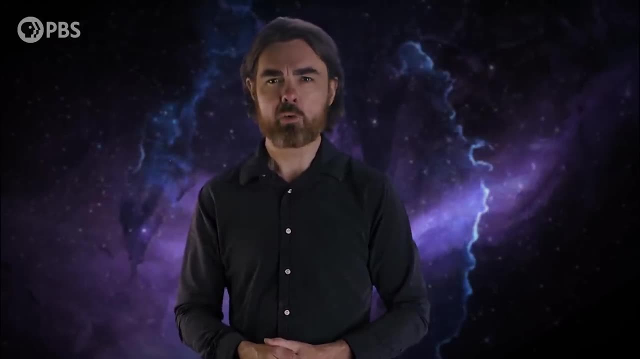 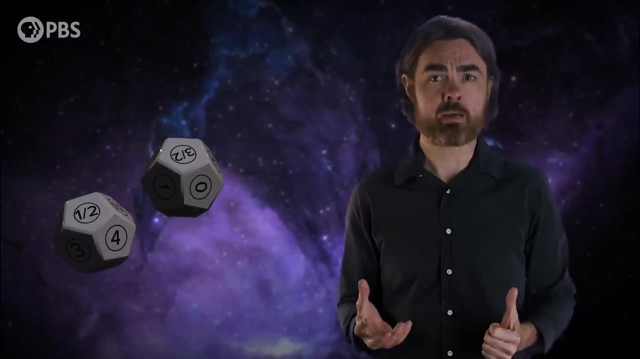 an extended, although still tiny region. However you explain it, we have an excellent working description of how spin works. We say that particles described by spinners have spin, quantum numbers that are half-integers, Half 3 on 2,, 5 on 2, etc. The electron itself has spin. 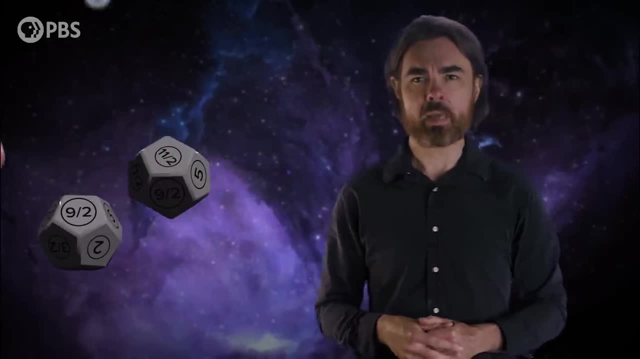 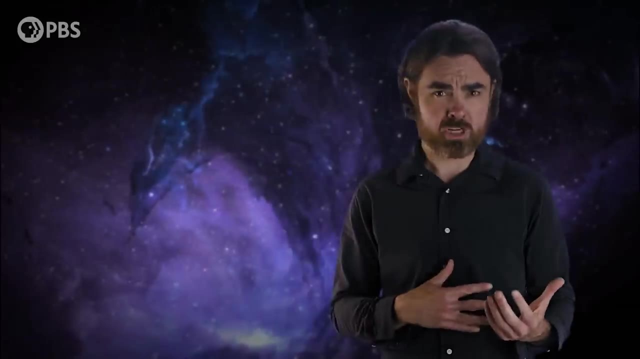 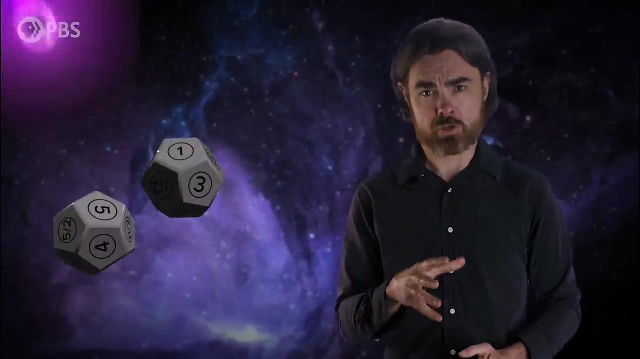 half. So does the proton and the neutron. Their intrinsic angular momenta can only be observed as plus or minus a half-integre. We call these particles fermions. Particles that have integer spin are called bosons and include the force-carrying particles like the photon. 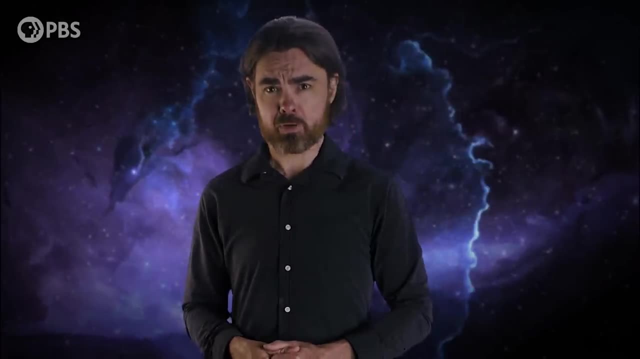 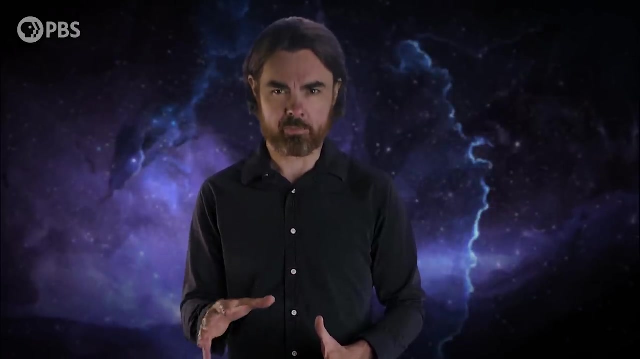 the gluon, etc. These are not described by spinors, but instead by vectors and behave more intuitively. A 360-degree rotation brings them back to their original state. This difference in the rotational properties of fermions and bosons results in: 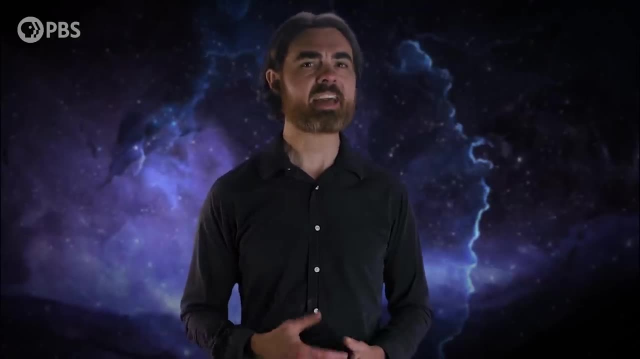 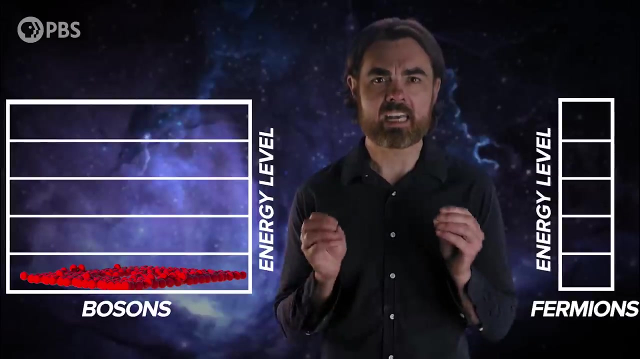 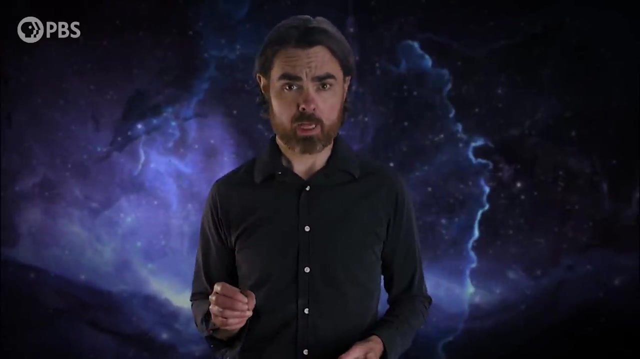 profound differences in their behavior. It defines how they interact with each other. Bosons, for example, are able to pile up in the same quantum states, while fermions can never occupy the same state. This antisocial behavior of fermions manifests as the Pauli exclusion principle. 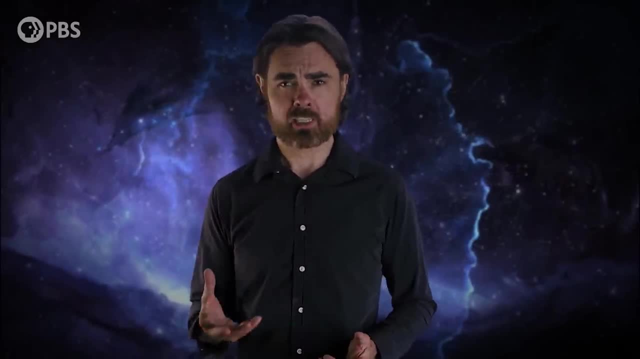 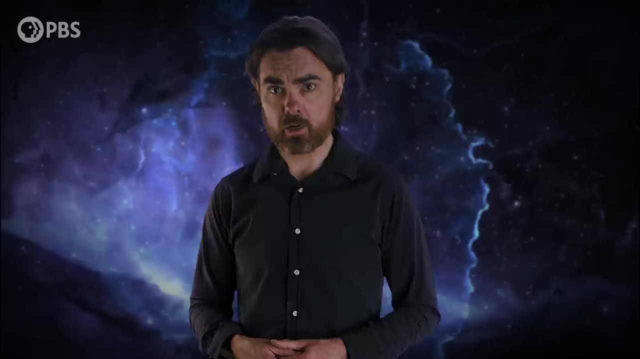 and is responsible for us having a periodic table for electrons living in their own energy levels and for matter actually having structure. It's the reason you don't fall through the floor right now. But why should this obsess? Why should an obscure rotational property lead to such fundamental behavior? 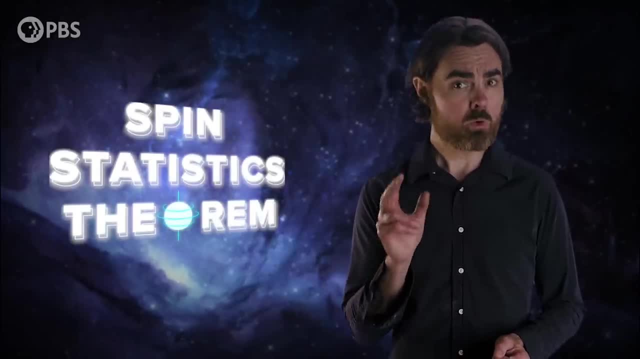 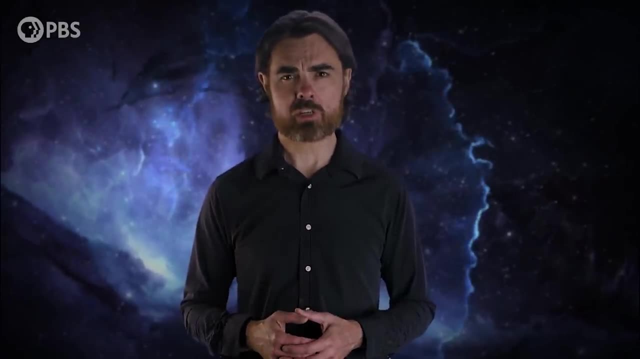 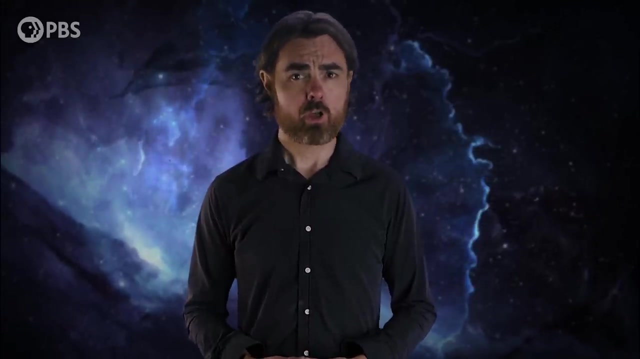 Well, this is all part of what we call the spin statistics theorem, which we'll come back to in an episode very soon. Electrons aren't spinning, They're doing something far more interesting. The thing we call spin is a clue to the structure of matter, and maybe to the structure of reality. 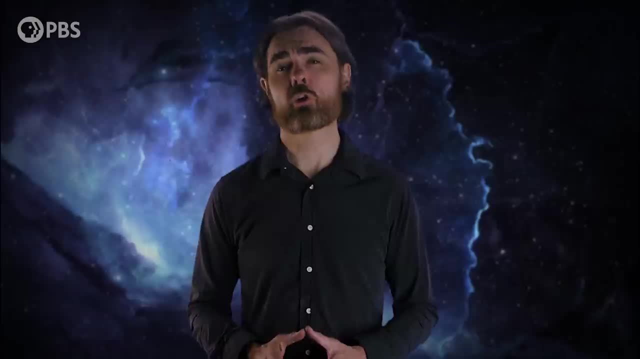 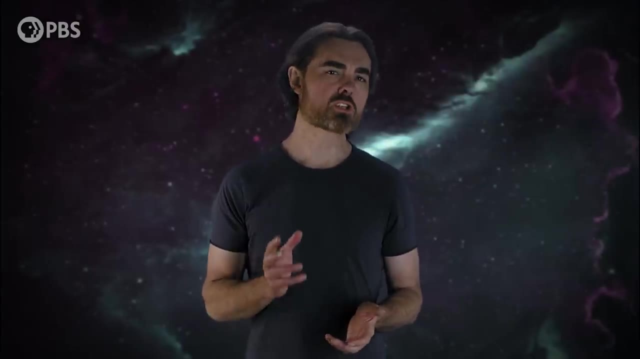 itself through these things that we call spinors, strange little knots in the subatomic fabric. Last time we talked about the connection between quantum entanglement and entropy. This was a heady topic, to say the least, but you guys had such incredibly insightful comments and 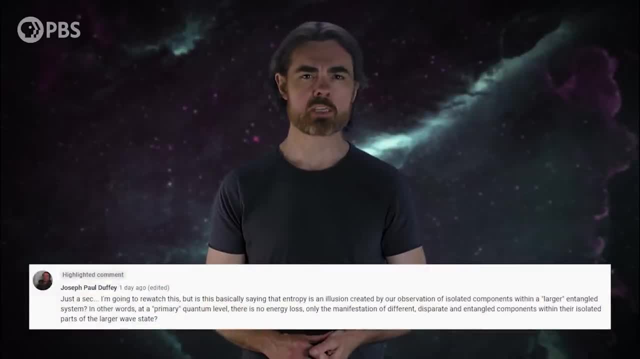 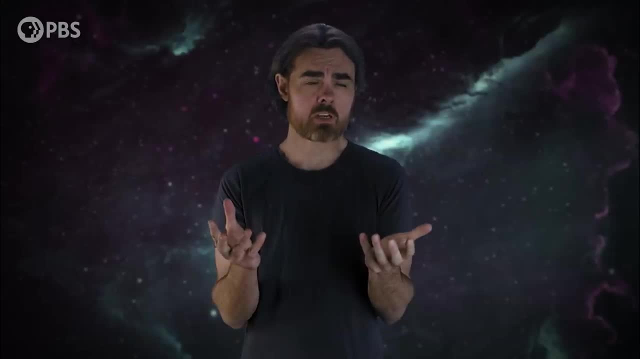 questions. Joseph Paul Duffy asked whether entropy is an illusion created by our observation of isolated components within a larger entangled system. Well, the answer is that entropy is sort of relative. It's high or low depending on context. The air in a room may be perfectly mixed. 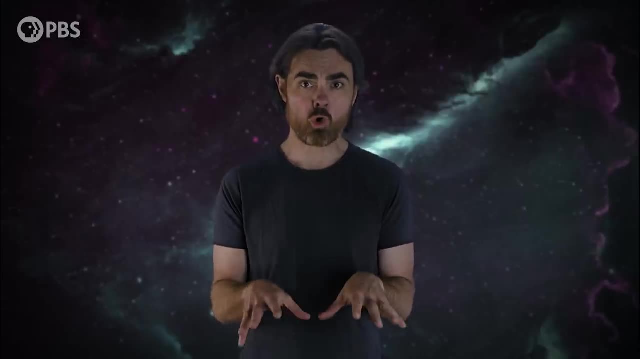 and so considered high-entanglement. The air in a room may be perfectly mixed and so considered high-entanglement, but if that room is warm compared to a cold environment outside, then the total environment in a room is at a relatively low entropy. 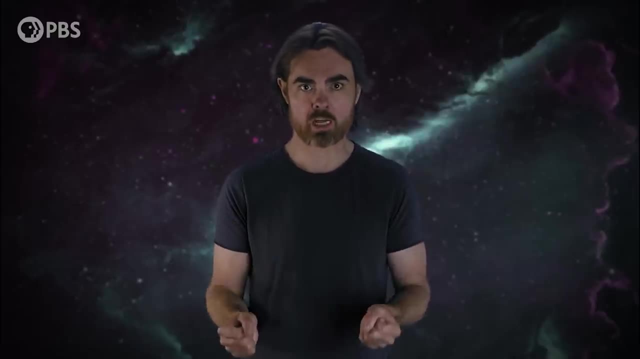 compared to the maximum if you let the temperature equalize. Von Neumann entropy is different to thermodynamic entropy in that it represents the information contained in the system and extractable in principle, versus information that is lost to the system by entanglement with the environment. On the other hand, classical or thermodynamic entropy, 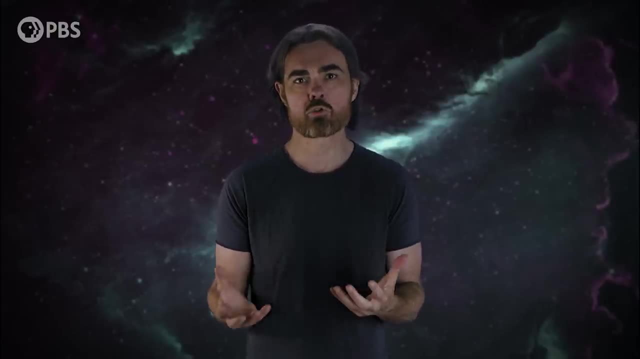 dynamic entropy represents information that is hidden beneath the crude properties of the system, but may in principle be extracted. And yet von Neumann entropy has a similar contextual nature. If your system has no entanglement with the environment, then its von Neumann entropy is. zero, but if you consider a subsystem within that system, then the entropy rises. Randomated asks the following: If entropy only increases over time, which implies it was at its minimum at the big bang, does that mean there was no quantum entanglement at the big bang? 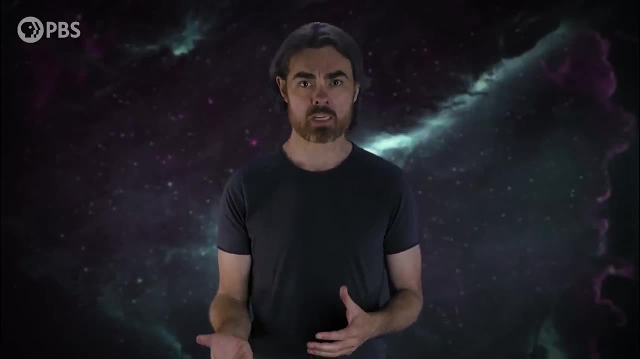 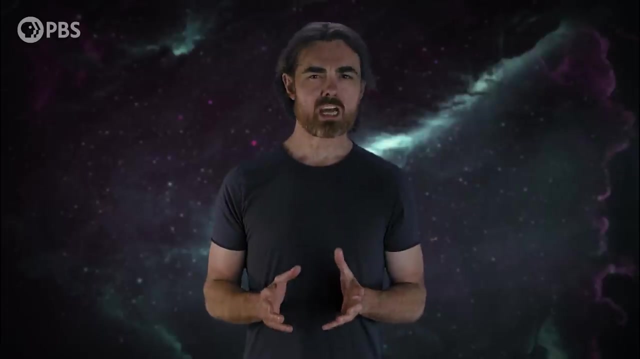 Well, to answer this, we'd need to know why entropy is so low at the big bang, and that's one of the central mysteries of the universe. But I'll give it a shot anyway. So we can't really talk about the t equals zero beginning of time, because that moment 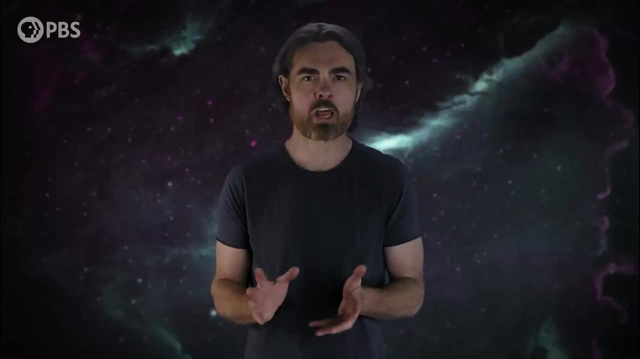 is lost in our ignorance about quantum gravity and inflation and whatever other crazy theory we haven't figured out yet. But what we do know is that the t equals zero. beginning of time is zero. What we do know is that at some very, very small amount of time after t equals zero, the 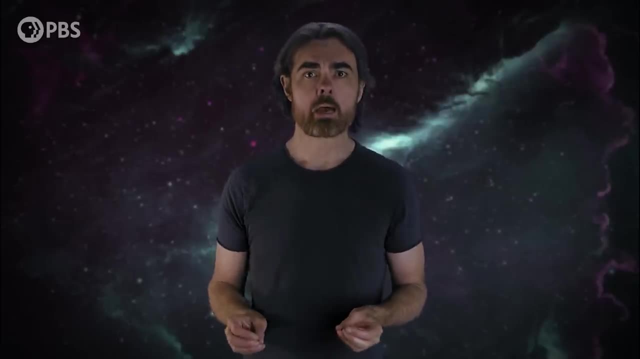 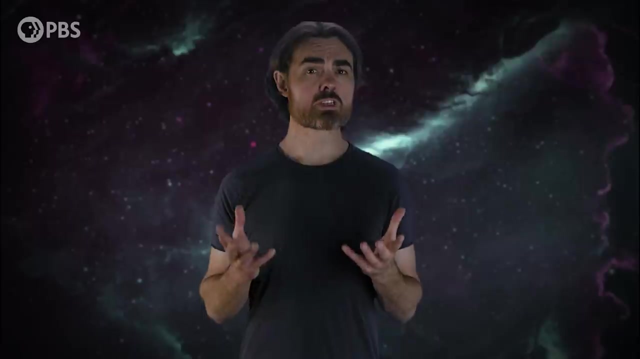 universe was extremely compact, which meant hot and dense, and was also extremely smooth. The compact part is where the low entropy comes from. The gravitational degrees of freedom were almost entirely unoccupied. On the other hand, the extreme smoothness meant that the entropy associated with matter 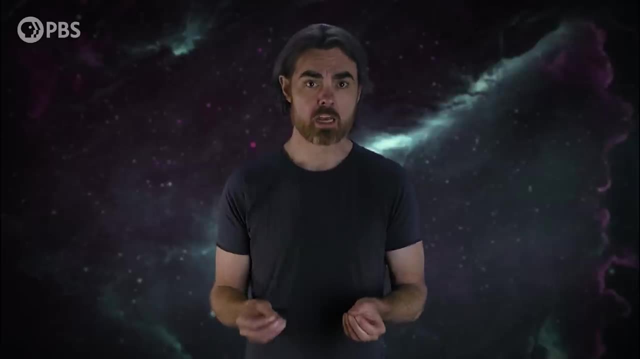 was extremely high. Energy was spread out as it could get between all of the particles and the different ways they could move. The low gravitational entropy massively outweighed the matter entropy, so entropy was low. That smoothness, though, seems to suggest that the particles of the early universe were 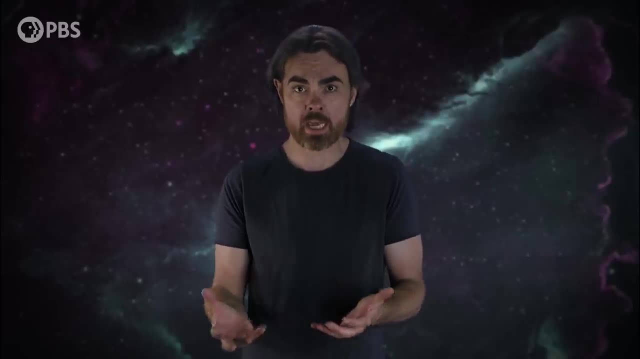 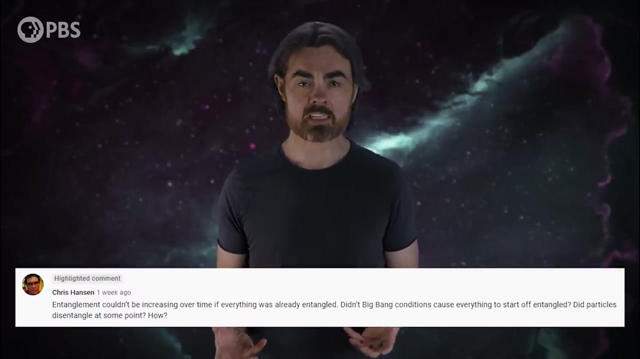 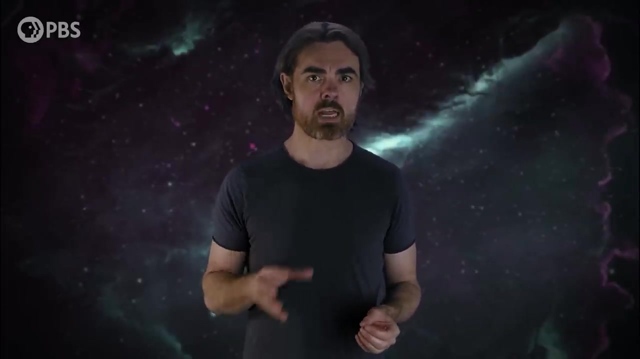 already entangled, otherwise how did they spread out their energy? Chris Hansen makes the same point, asking if the conditions of the big bang meant everything started out entangled. Well, you'd think so, but that's not necessarily the case. Remember that von Neumann entropy is relative to the energy of the universe. 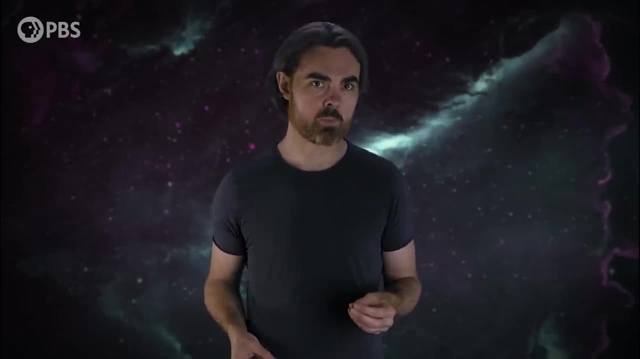 It is relative to the system you're talking about, and so is entanglement. Let's say you have a bunch of particles that are not entangled with each other but are entangled with another bunch of particles somewhere else. If you ignore those other particles, then it seems like there's no entanglement in.